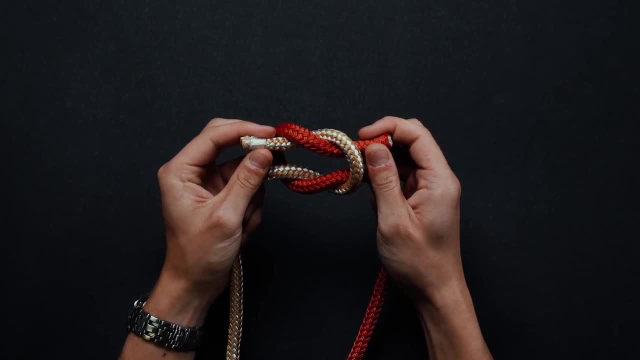 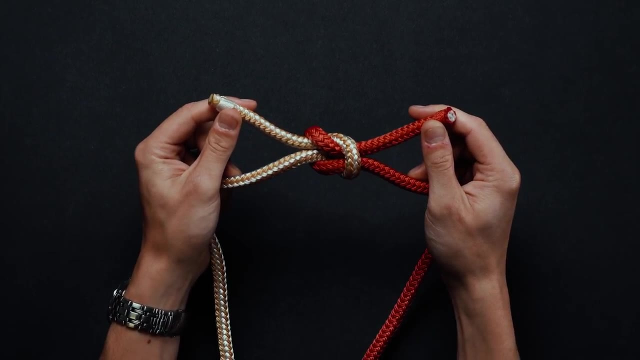 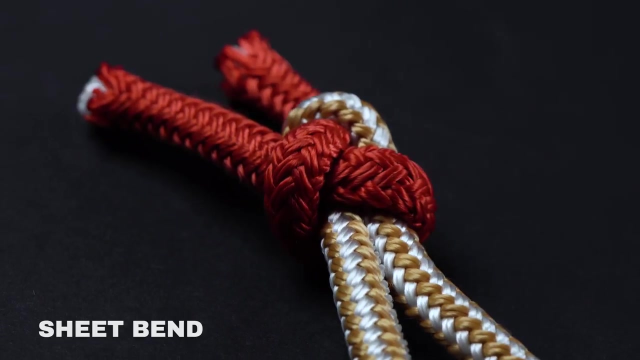 your left hand To tighten. pull the running ends away from each other. at the same time, You've now completed a square knot. If you've tied your knot correctly, each end will be running parallel to its respective length of rope. Similar to a square knot, the sheet bend is best used for tying two lengths of rope together. 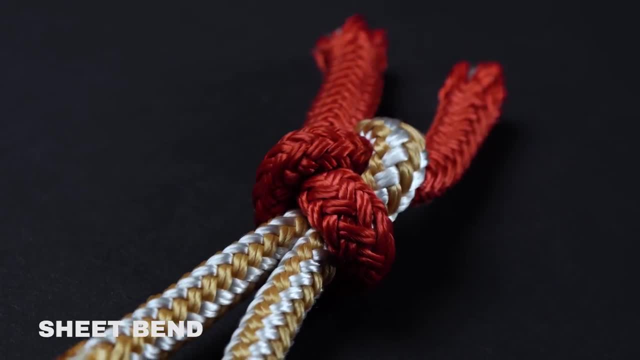 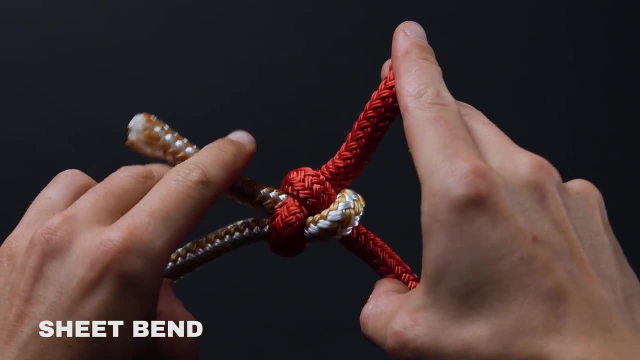 especially if they happen to be of different sizes or materials. As such, sheet bends are also known as weaver's knots when used with yarn or twine. It's worth noting that for a sheet bend to have any strength, the two free ends should. 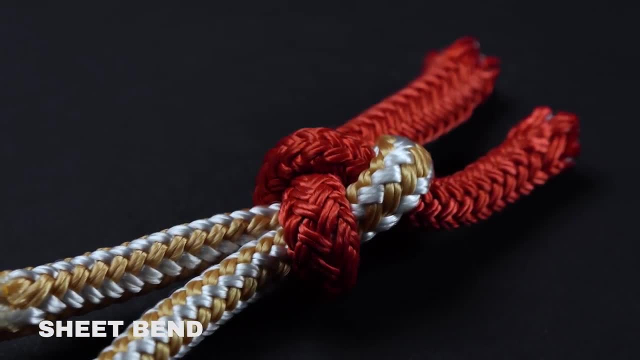 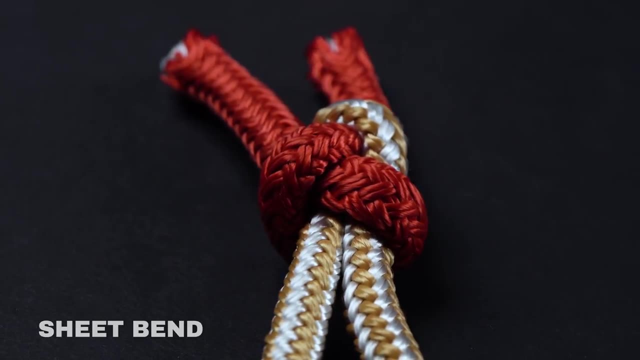 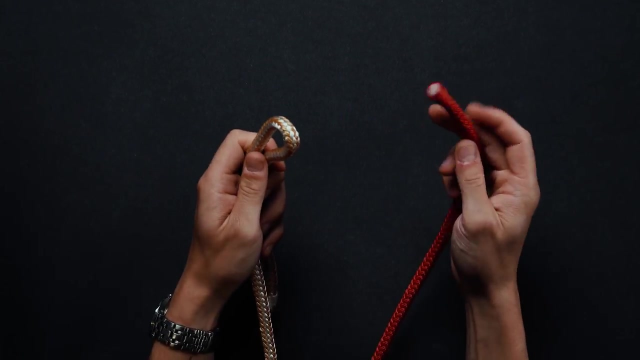 line up on the same side of the knot. If they happen to be on opposite sides, a left-handed sheet bend, the knot will slip under load and release completely. Let's get to it. Begin by forming a loop using the end of one rope. Bring the free end of your second joining. 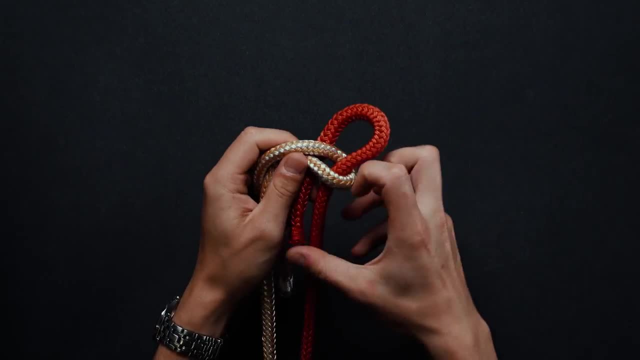 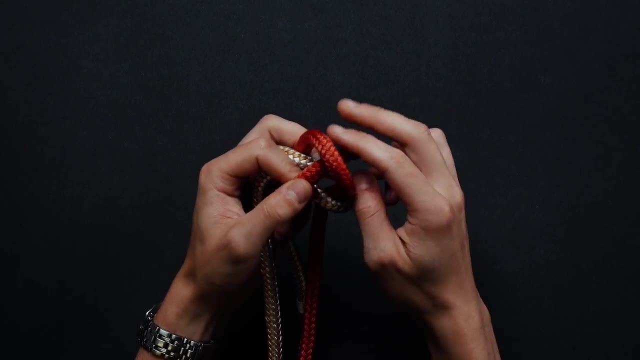 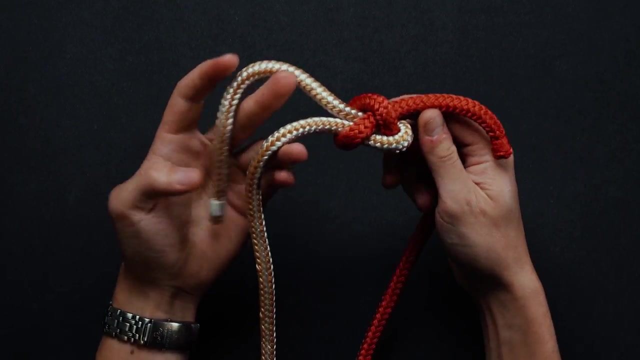 rope under and through the opening of the loop. Wrap the joining rope around both ends of the looped rope. Pull the joining rope under itself. Complete the knot by pulling all four ends to tighten. You have now completed a sheet bend. You can perform a double. 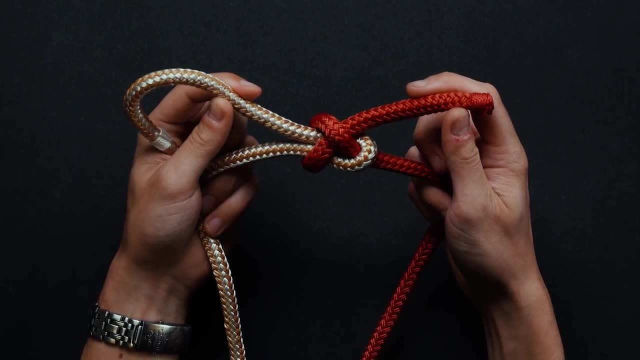 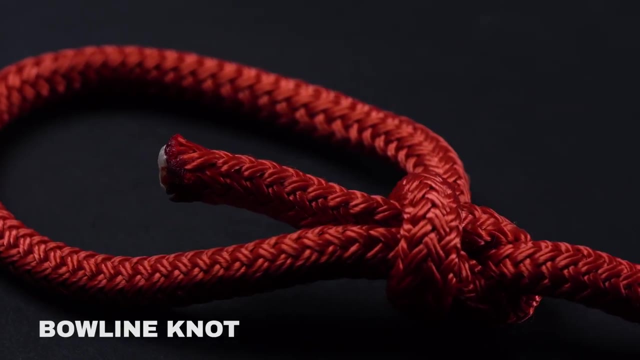 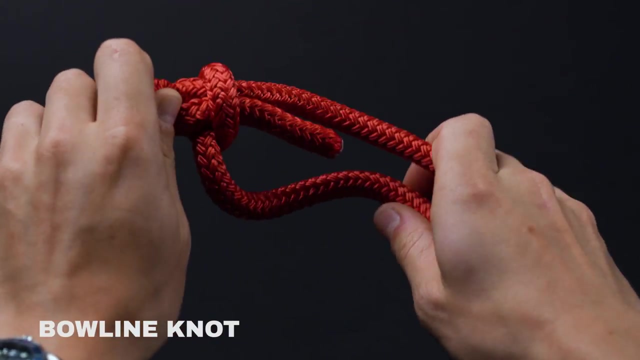 sheet bend by wrapping the joining rope around the looped rope for a second time. Bow lines are easily amongst the most useful types of knots you can know. They've been used for centuries on account of their reliability, stability and strength. Commonly used for forming a fixed loop at the end of a rope, they're 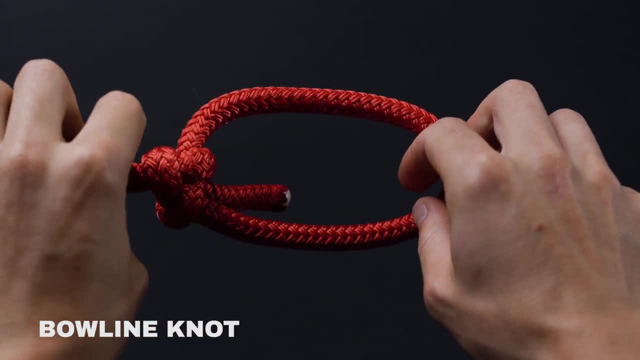 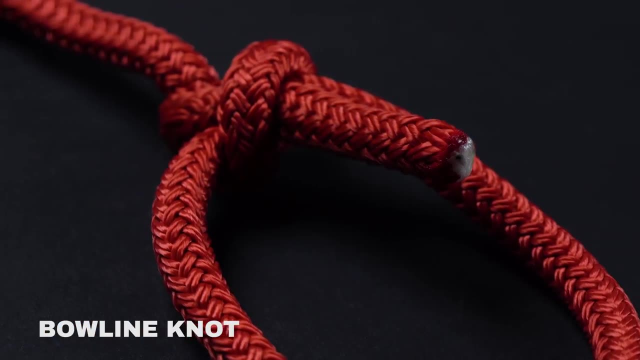 highly secure, yet still plenty easy to untie. Accordingly, you should never use a bow line in critical life-or-death applications. Sure, it bites far better than other types of knots, but it only maintains about 60% of the rope's. 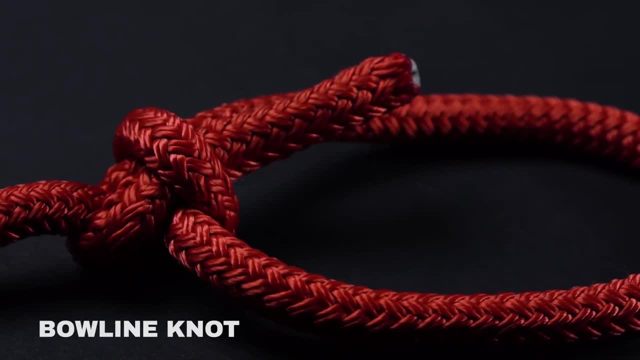 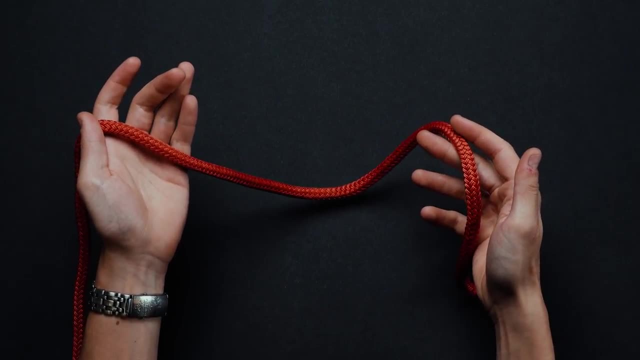 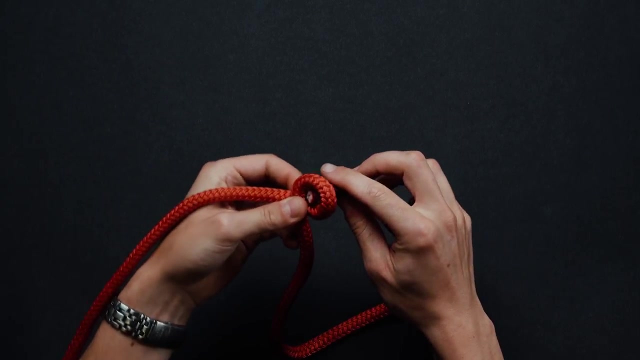 overall strength. With this in mind, it's time to get tying An. initiate the knot by draping the rope across one hand, with several inches of the free end hanging down. Form a small loop. with the rope in your hand, Bring the free end back up, Pass it through the underside of the loop, Continue around. 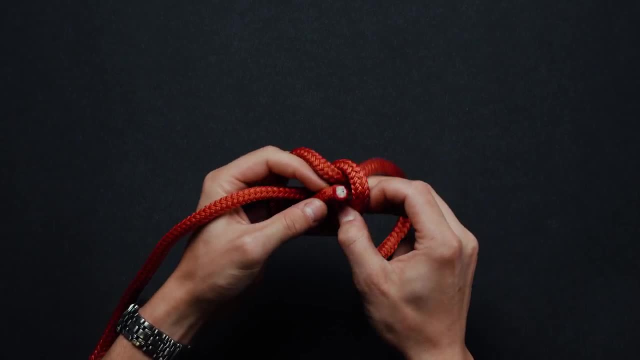 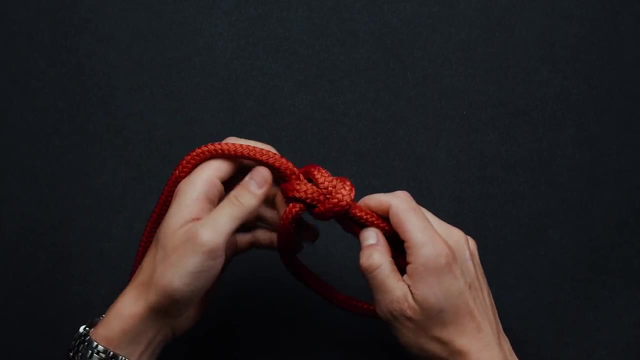 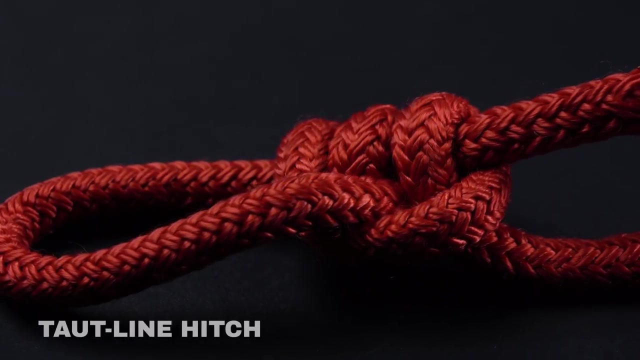 the backside of the standing rope segment. Pull the free end down through the same loop that you just came through Tighten. by holding the standing line and pulling on the free end, You have just completed a bowline In scenarios where you might need to tie an adjustable sliding knot on your rope. the 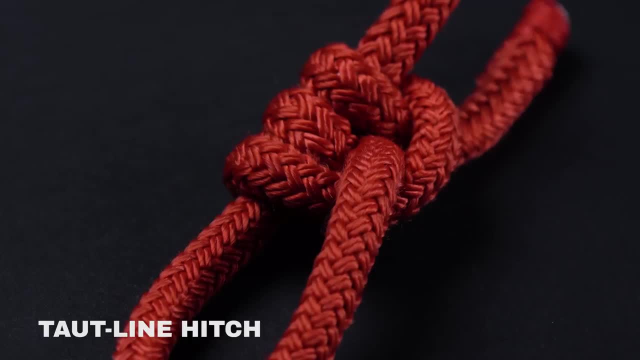 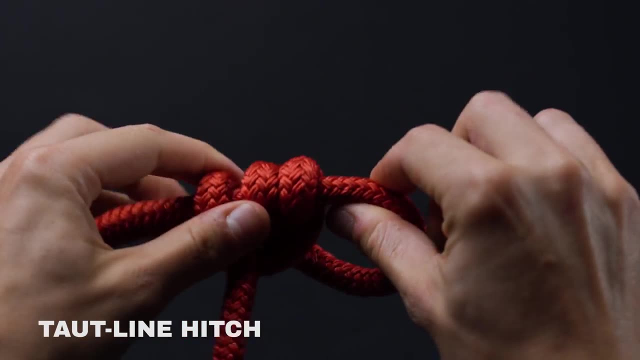 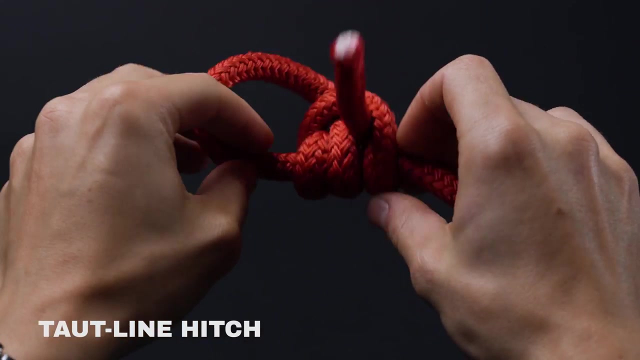 Boy Scouts of America recommends the tautline hitch. Perfect for securing guylines and other supportive rope segments. it's a free-moving knot that bites hard and jams when placed under load. As such, the tautline hitch is an incredibly versatile tie that's commonly used on everything. 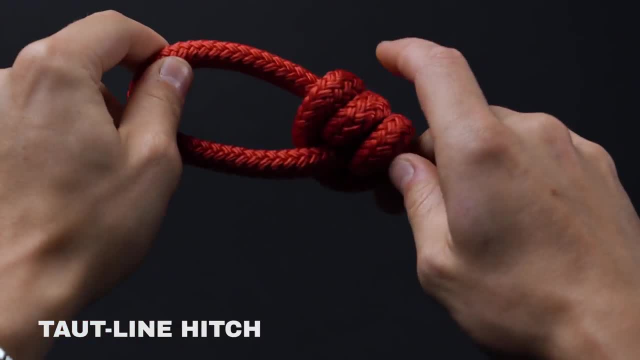 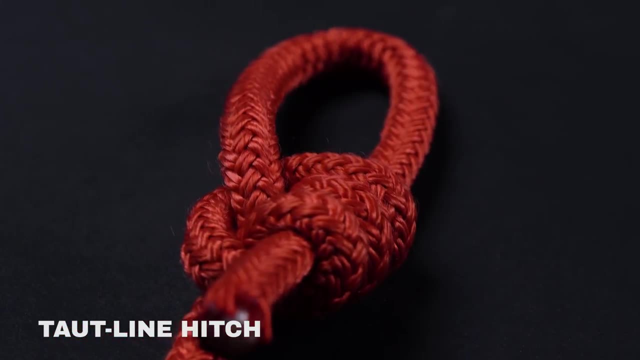 from aircraft to adjustable moorings. In fact, you can tie the tautline hitch to any of your favorite hoops. It's such a trusted knot that astronauts even used it when repairing the Hubble Space Telescope aboard the STS-82 mission. 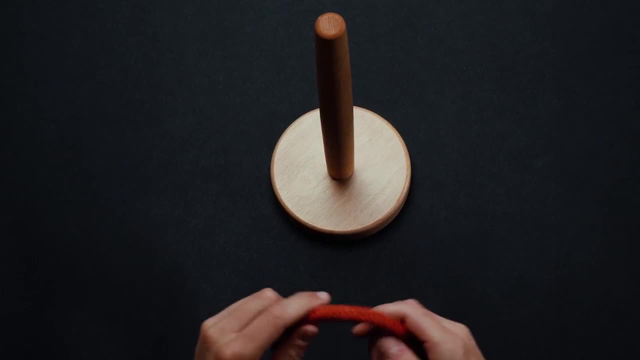 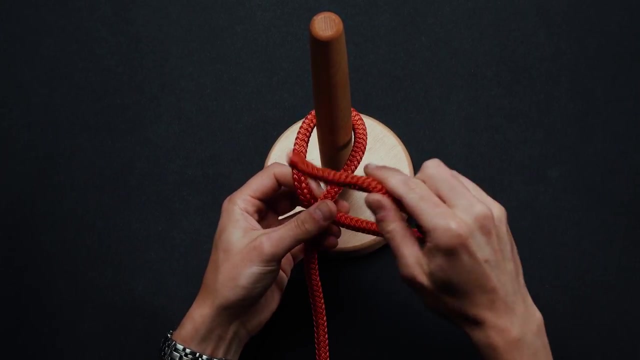 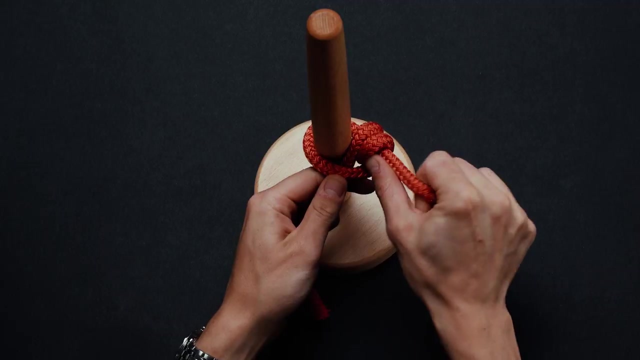 Let's begin. Take a generous length of rope and bring it around a post or similar object. Pass the free end under the standing segment and between the two sections of rope. Repeat once more, working toward the post. Coil the free end under and around the standing line above. 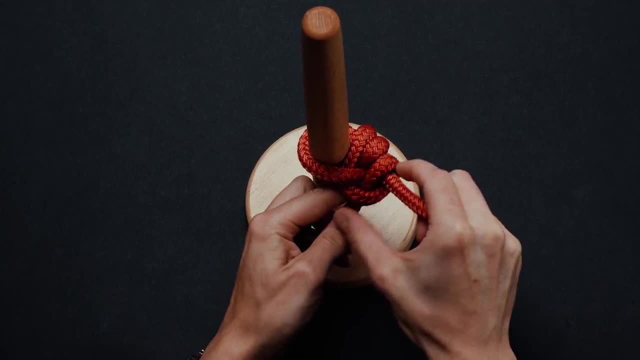 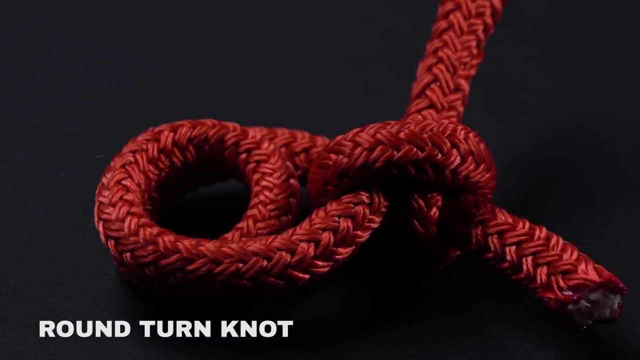 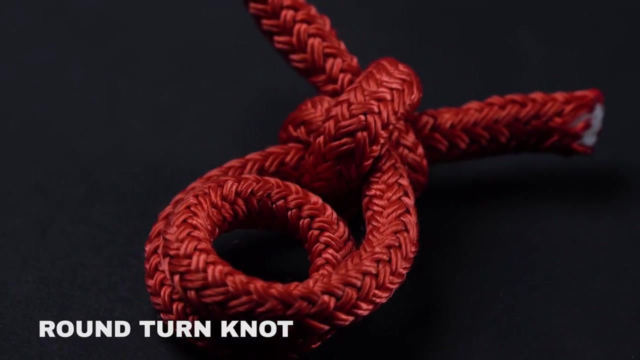 the coil. Tighten the knot by pulling on the free end. You have now completed a tautline hitch. The round turn and two half hitches is a knot that's used to attach the end of a rope to a fixed object Made up of two parts. the turn bears the brunt of the load, while the 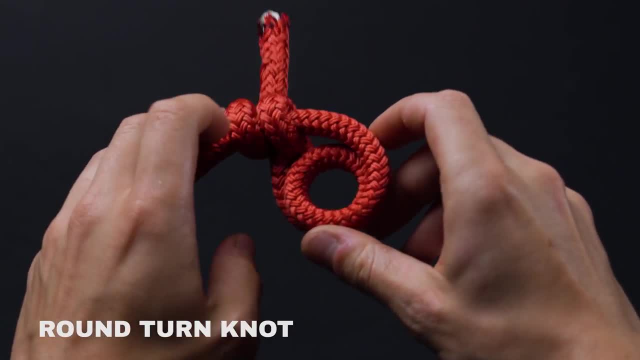 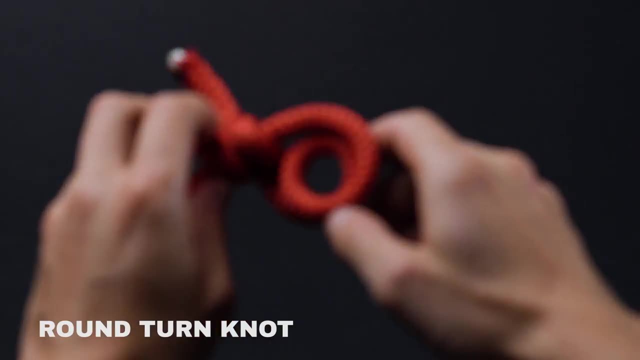 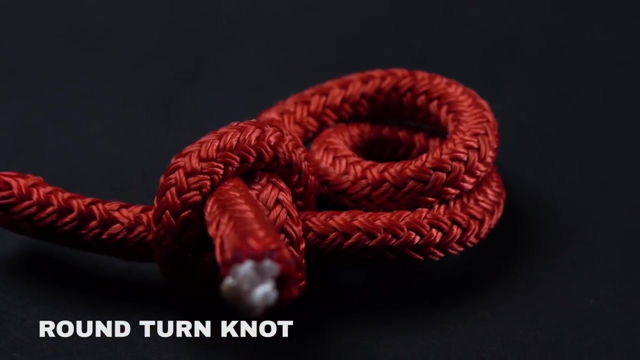 hitches provide additional support. In conjunction, they allow the knot to retain as much as 75% of the line's overall strength. One of the primary benefits of the round turn is that it can be tied and untied when under load. Moreover, it's highly unlikely that the knot 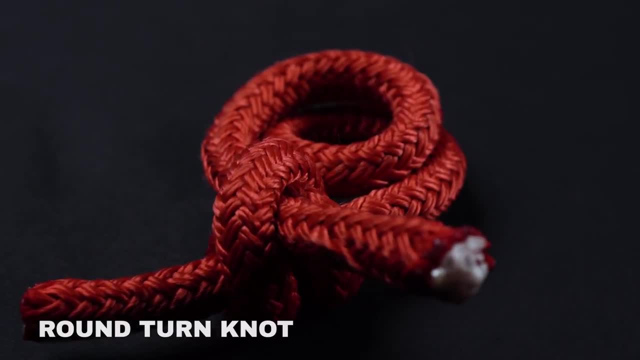 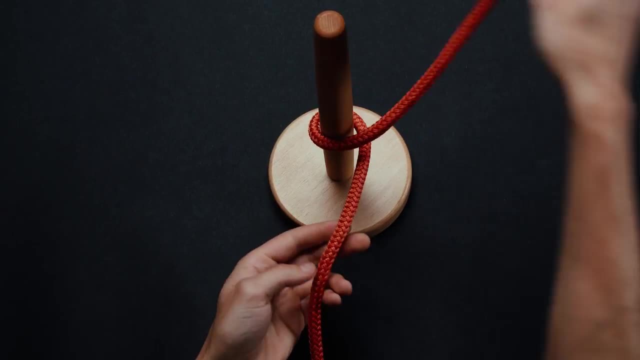 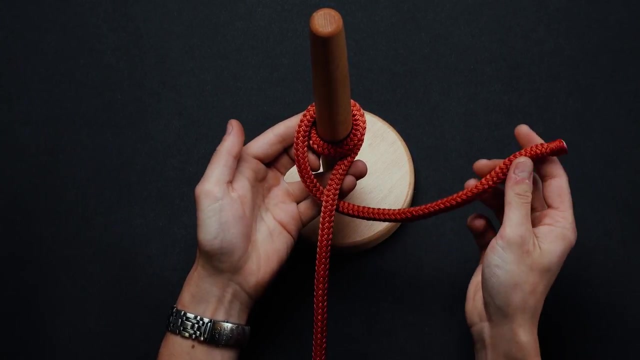 will ever slip and you never have to worry about it jamming. Now onto the knot. Begin by bringing one end of the rope under and around your object of choice Twice. Pass that same working end underneath the standing end, Make a turn and pull the rope. 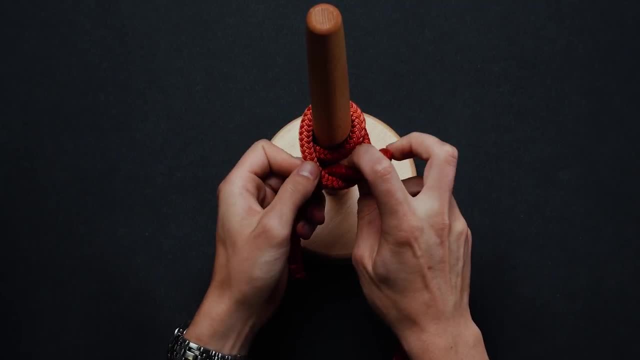 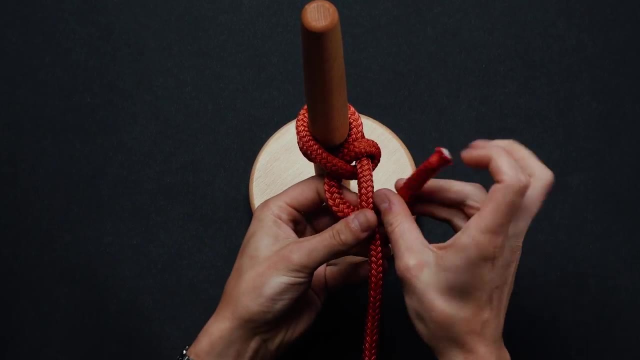 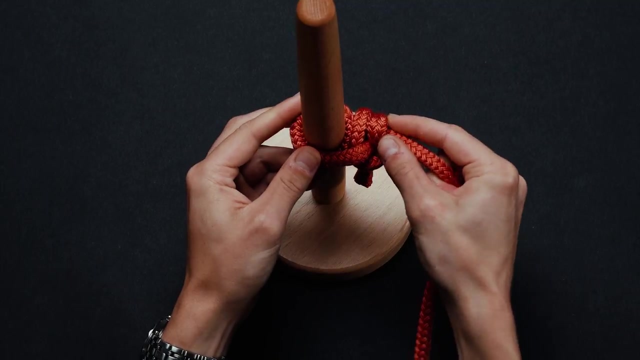 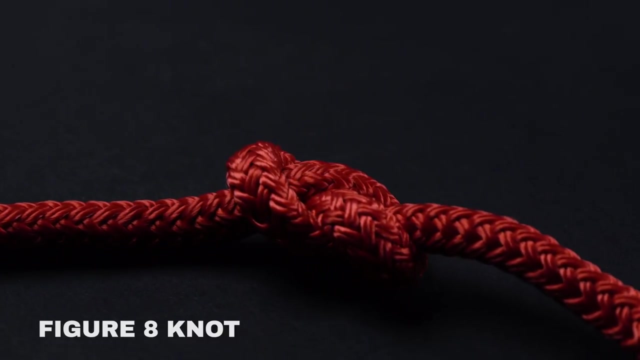 through the loop. you just made Cinch it tight. Repeat steps three and four. You have now completed a round turn and two half hitches. If you'd like to further secure your knot, you can add additional half hitches. Up until now, our knots have been primarily intended for attachment, be it to another. 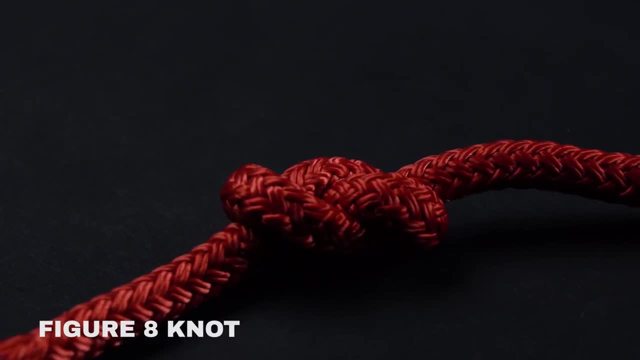 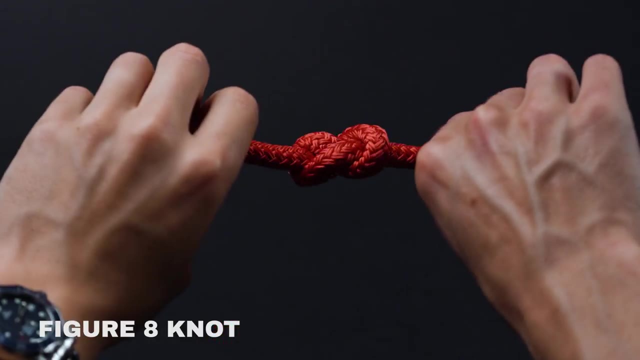 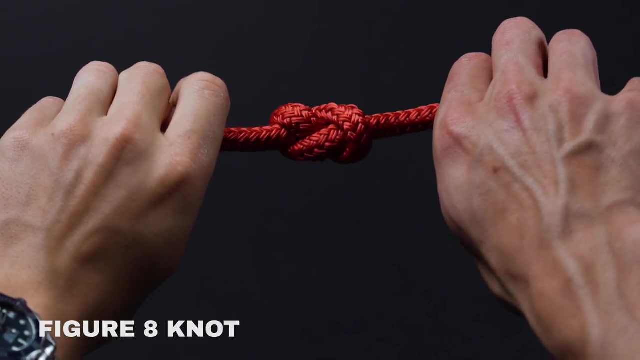 length of rope or a different object altogether. The figure eight knot, however, is a knot that's used to prevent ropes from slipping out of retaining devices. Accordingly, it's a knot that's ubiquitous throughout climbing and sailing, Because the figure eight knot maintains about 80% of the rope's overall strength. it's 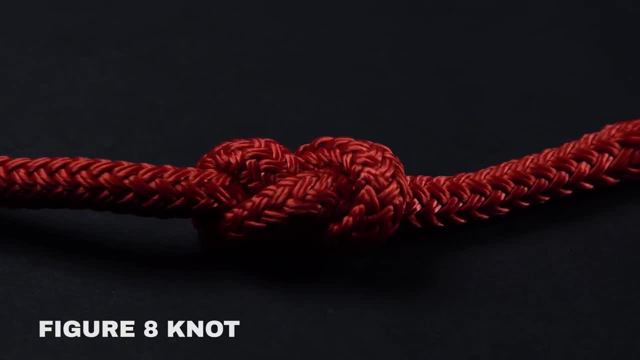 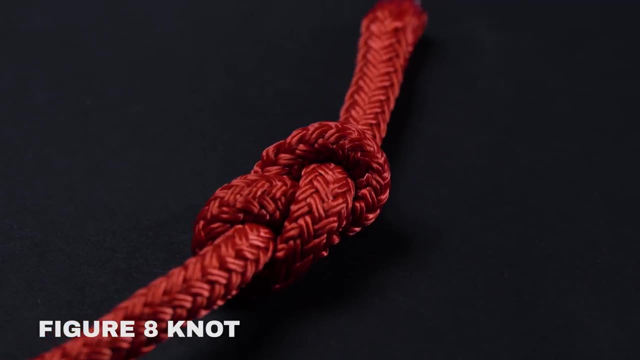 a knot that forms the basis of many other advanced ties, as it makes for an excellent foundation. Assuming you want even more security from your stopper, you can add a second pass to your figure eight and make it a double Without further ado. let's get started. 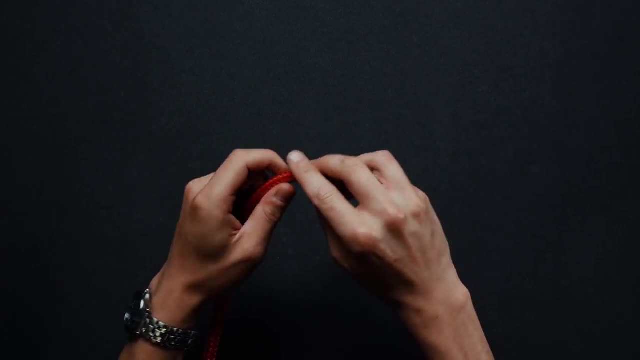 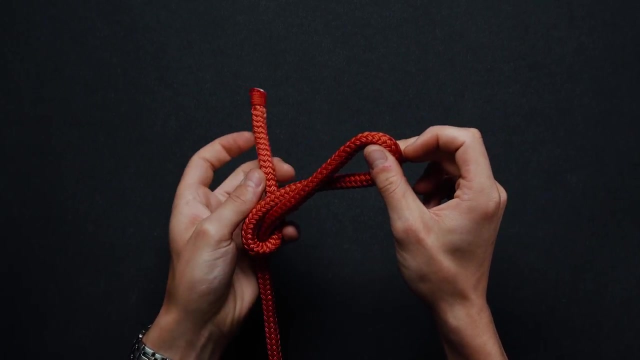 Make a loop with one end of the rope, bringing it under the standing segment. Complete the eight by bringing the working end over and under the standing end. Pull the working end through the loop you have created in step one. You have just finished your first figure. 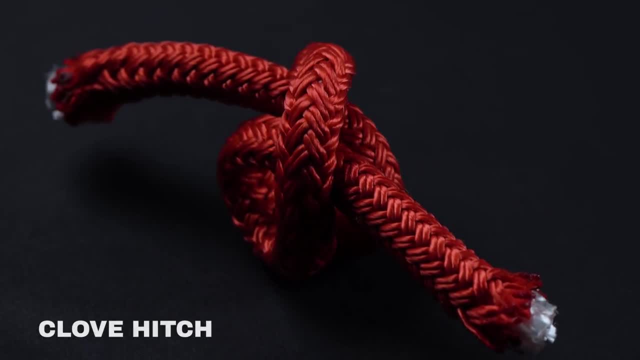 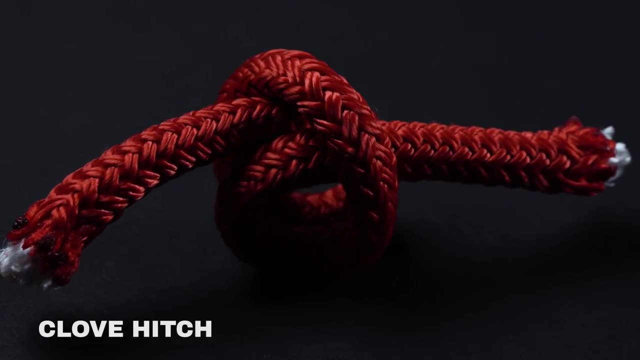 eight knot. While the clove hitch is by far one of the most useful knots you can learn, it's one that should only be tied in certain applications. That's because, for all of its ease and utility, the hitch can easily slip and or jam, depending on the gauge of the rope and the shape of. 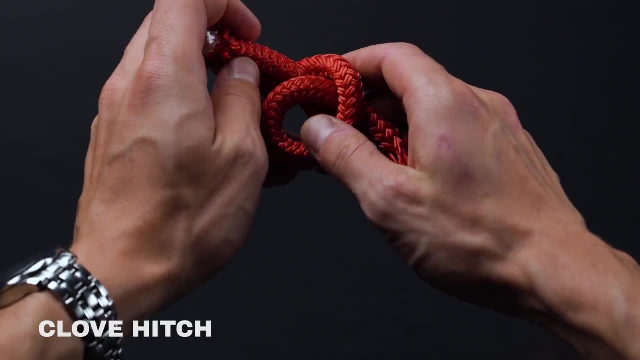 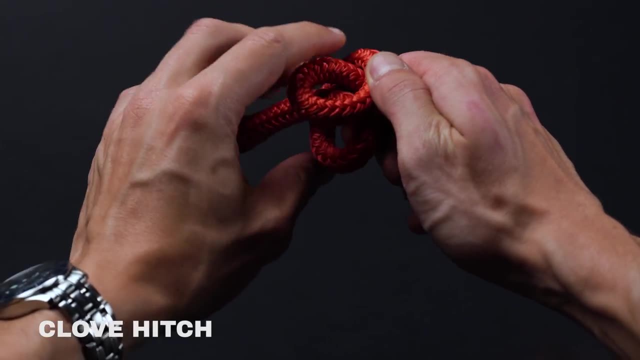 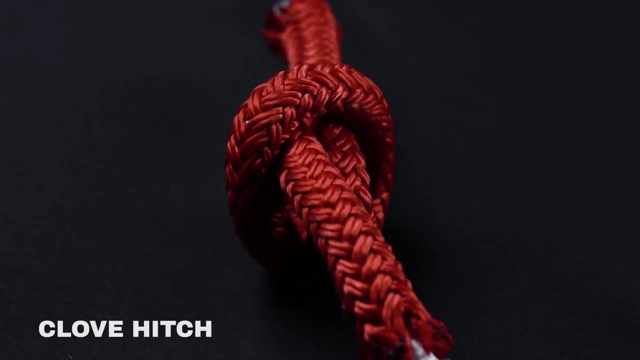 the object. As such, it's best to use a clove hitch in concert with half hitches and other more secure ties. It's worth noting, though, that adding too many secondary knots will often cause a clove hitch to bind. Thus, you should only use the knot in non-critical applications. 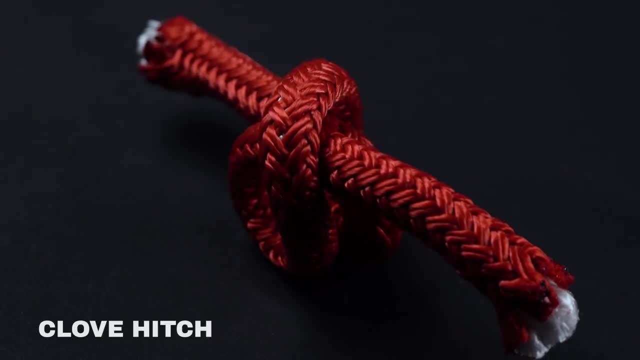 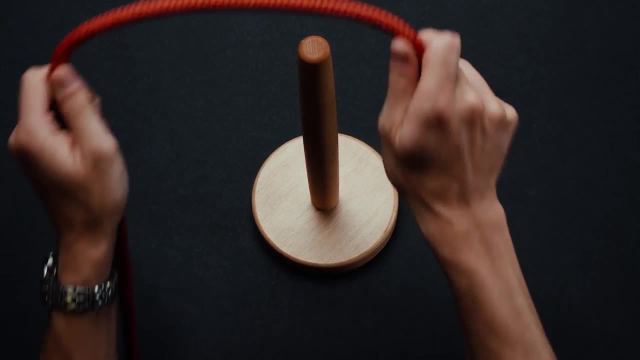 such as hanging a hammock or fixing a fender to a boat. Let's get started. Begin by wrapping the figure eight knot with the other end of the rope, bringing it under a free end of a rope, around a post or a similar object. Cross the rope over itself and around. 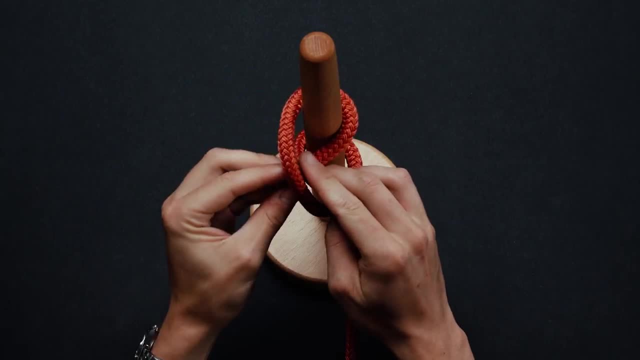 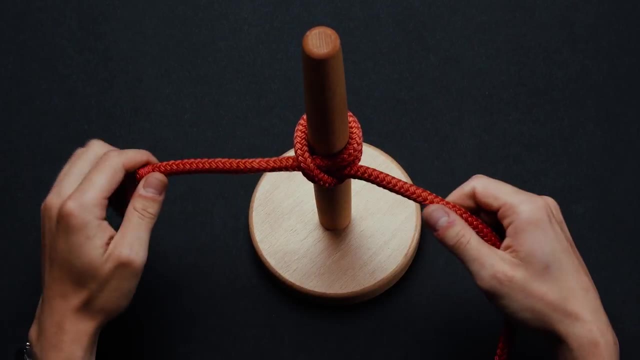 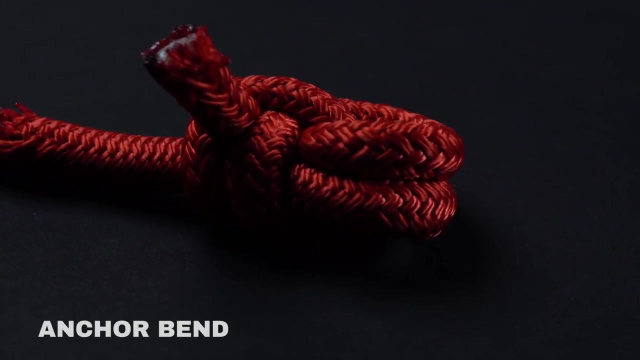 the post once more. Bring the working end under your last wrap. Pull to tighten, reducing excess looseness by cinching it up and down. You have now tied a clove hitch, As you'd expect. the primary function of the anchor bend is to attach lengths of rope to anchors. 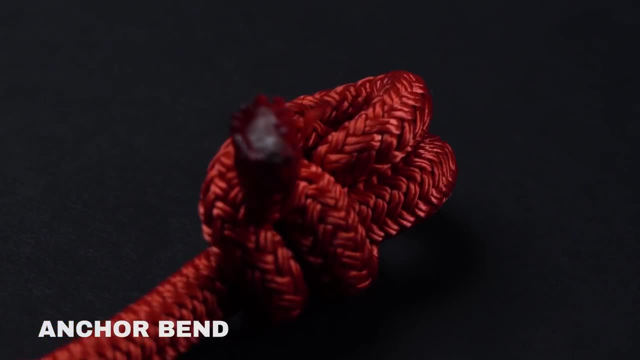 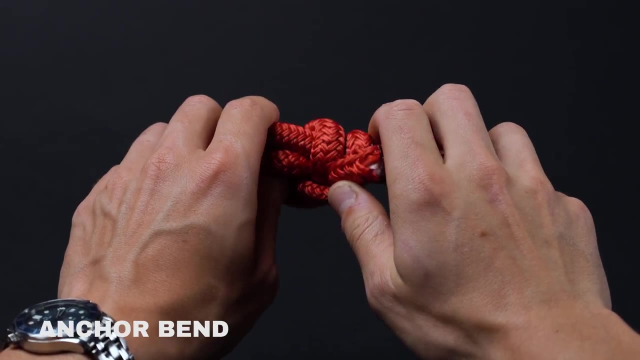 and other ropes. You can also tie a clove hitch to the end of the figure eight knot, as well as other ringed tie-offs. That being said, boating isn't the knot's only application. The anchor bend is also used by climbers when securing carabiners and by arborists when. 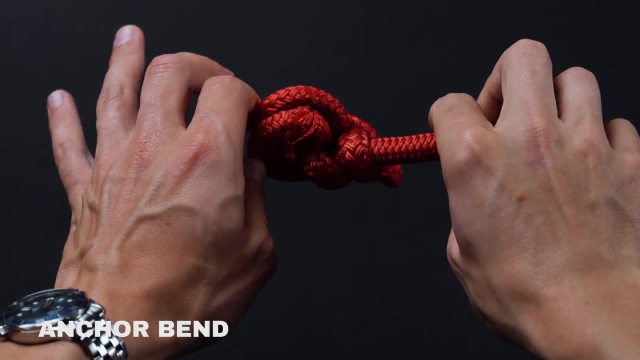 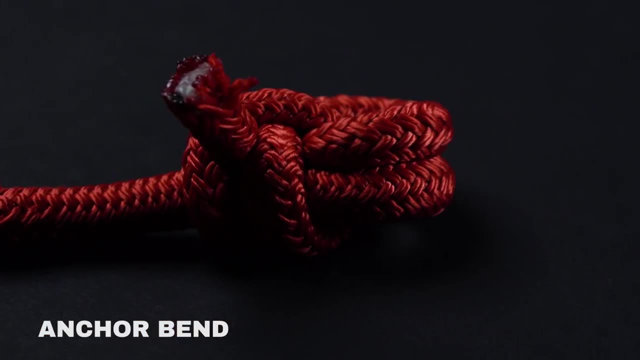 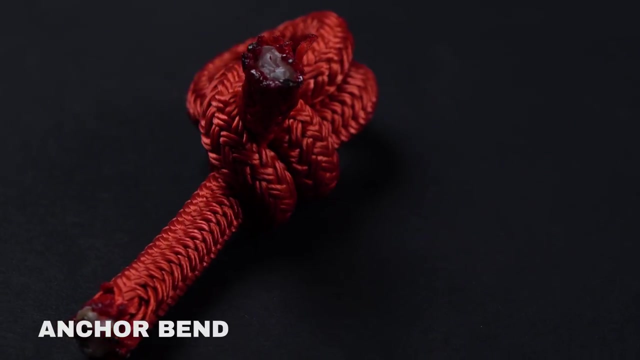 scaling trees. Interestingly, the anchor bend is very similar to a round turn and two half hitches, though one of the hitches is passed under the turn instead of over it, And the thing is, the knot is technically not a bend, It's actually a hitch. In any case, grab some. 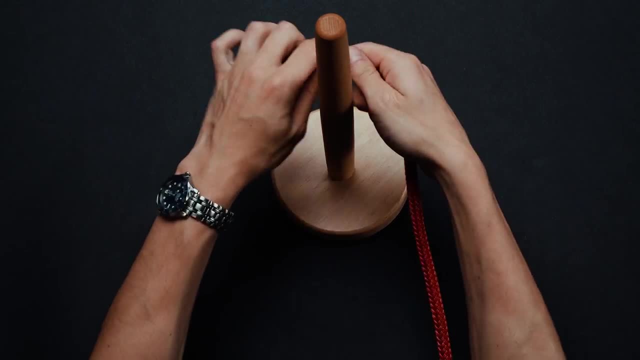 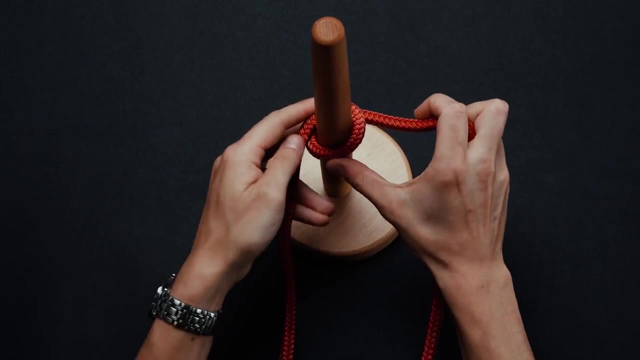 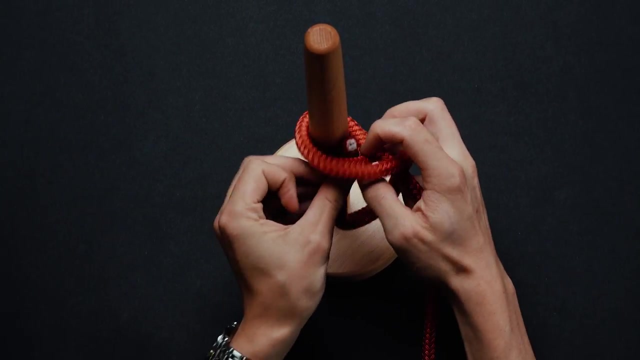 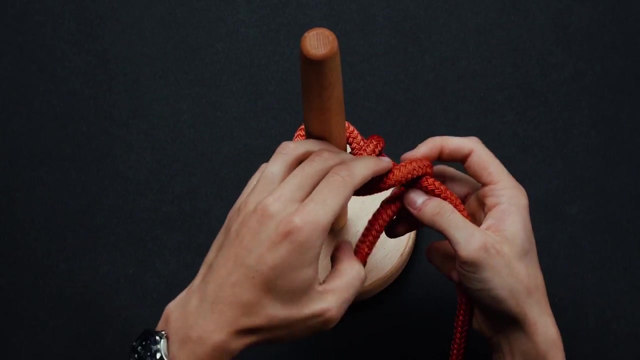 rope and get ready. Wrap your rope around your object two times, starting from the backside. Pull the working end over the standing segment. Wrap it around and pass through the loop made in step one. Pull tightly, Bring the working end over and back through the loop you've just made. Hold. 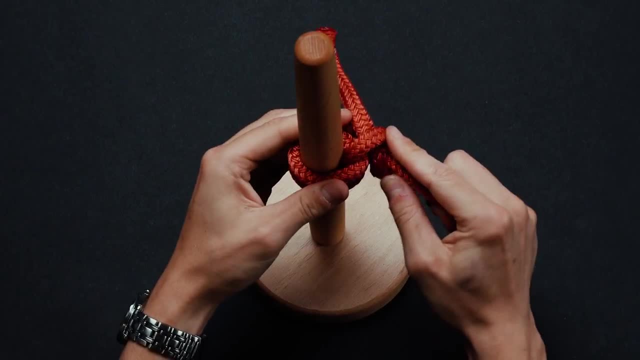 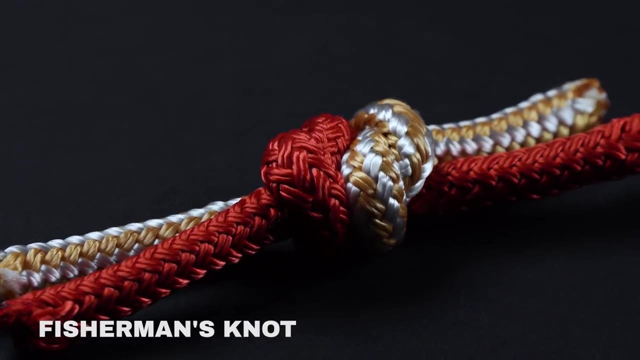 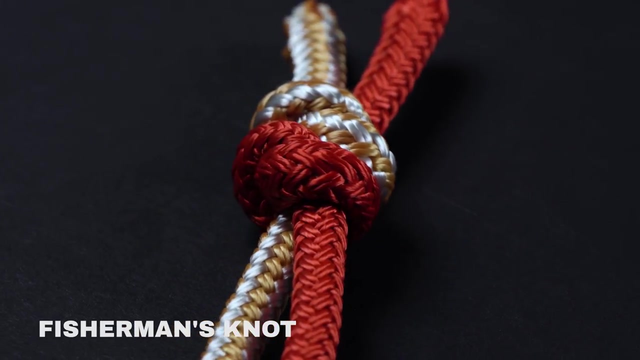 and pull tight. You have now completed an anchor: bend, Compact, strong and secure under strain. the fisherman's knot is best used for quickly tying two ropes of equal diameter together. Though the knot is rife with benefits, it can be cut very close and it's easily performed, even with wet hands. It weakens the rope with. 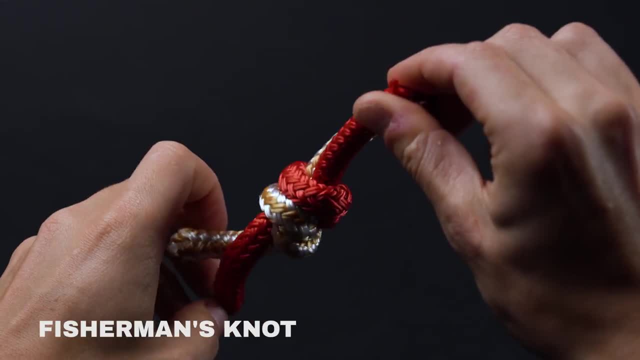 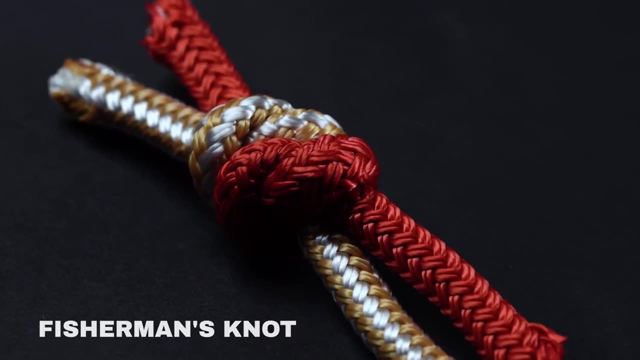 which it is tied. Should you be after an even more secure variation, you can switch up the knot with double overhand ties and altered overlappings, For that matter. you can even wrap the working end three or four times. You can also tie the knot with double overhand. 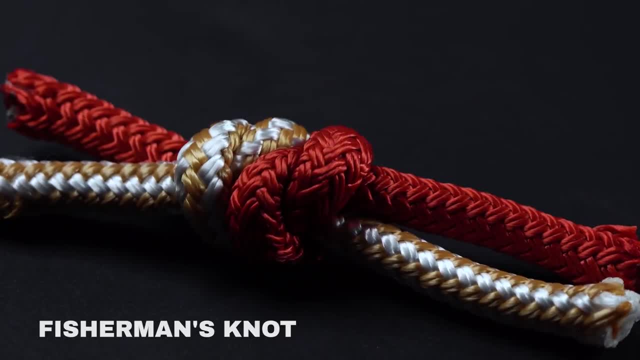 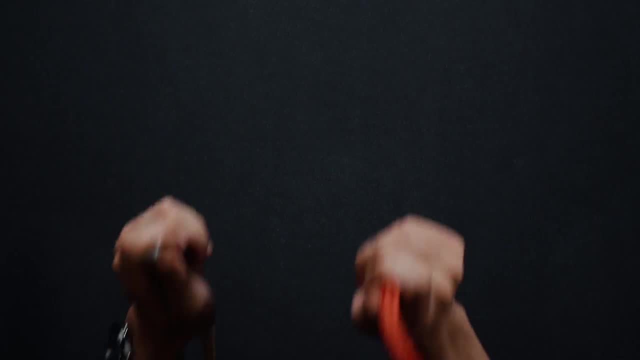 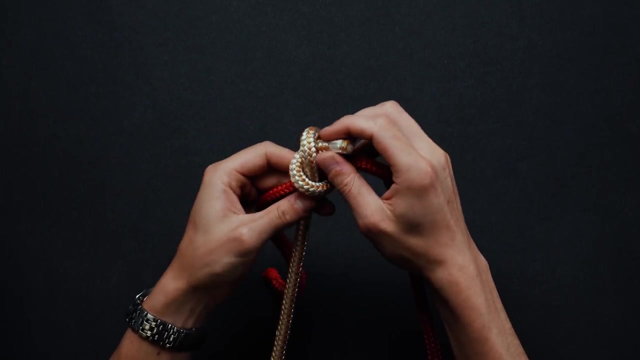 ties and altered overlappings. For that matter, you can even wrap the working end three or four times to ensure the utmost strength. Before we get ahead of ourselves, though, here's how to tie the fisherman's knot. Grab two lengths of rope. Tie a loose overhand knot with rope A around rope B. Do not tighten.